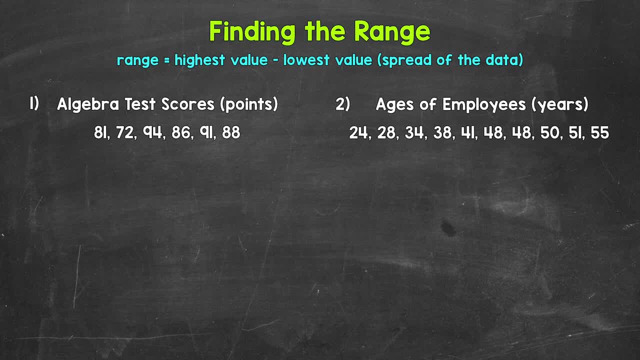 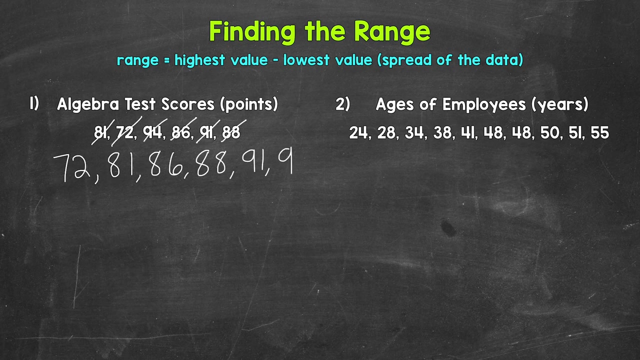 The lowest score is 72,, so that comes first, Then we have 81,, then 86,, then 88,, then 91, and then, lastly, 94.. Now that this data is in order from least to greatest, we need to find the range. We need to find the highest value and lowest value. 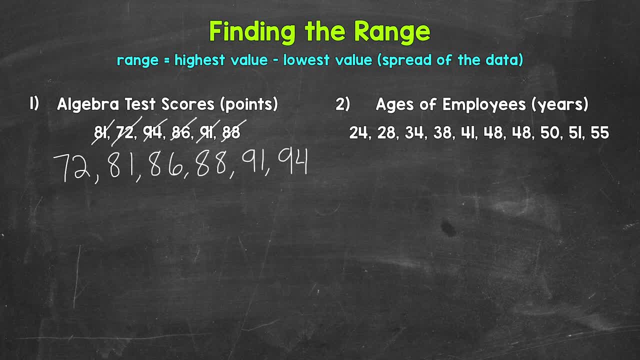 so the highest score and lowest score. The highest value is 94.. The lowest value is 72.. To find the range, we need to take the highest value, 94,, and subtract the lowest value, 72.. 94-72,. 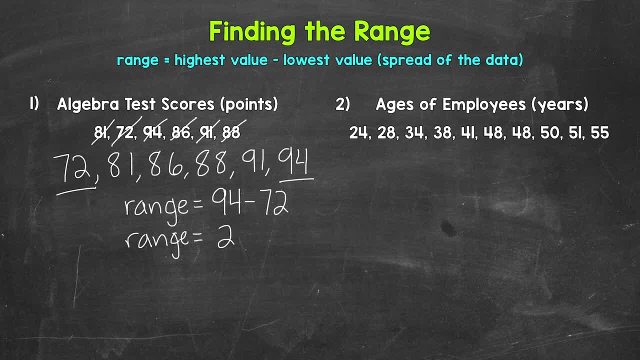 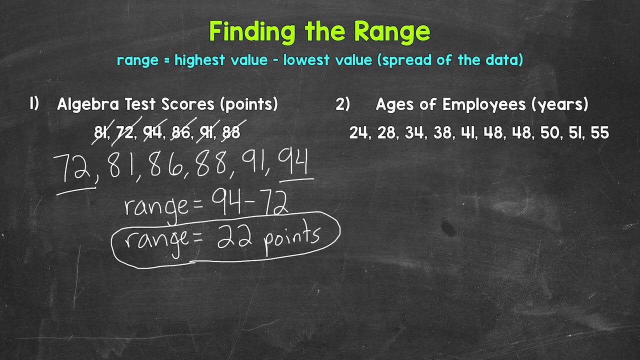 gives us a range of 22.. This is points, so we can label it. The range of these test scores is 22 points. That is the range of the data. The data goes from the lowest score, of 72 points, to the highest score of 94 points. 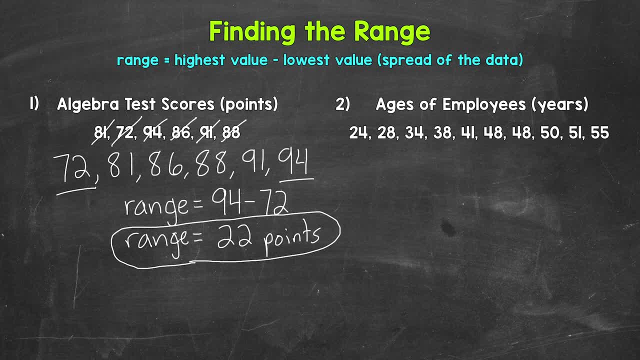 Again, the range is 22 points. is 22 points now when it comes to range. the higher the range, the greater the spread. so the data is more spread out. the lower the range, the data will be less spread out. for example, let's say that we: 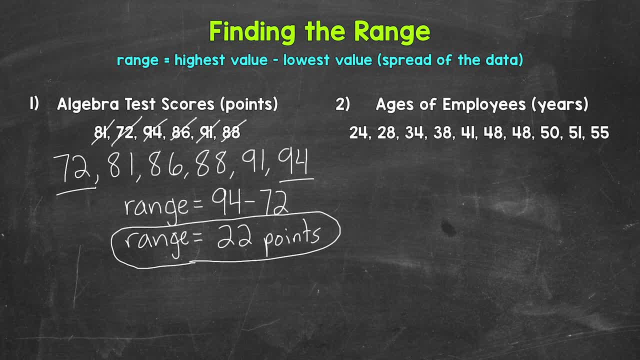 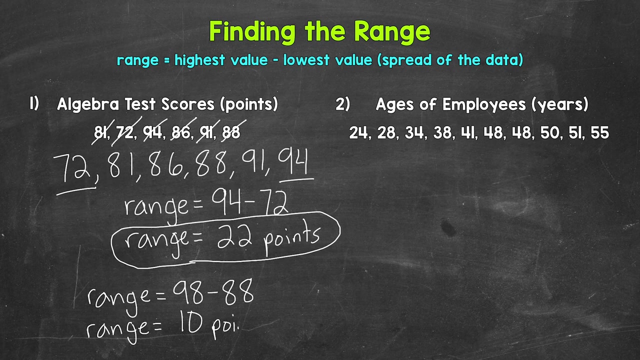 have another student where the highest score is 98 and the lowest score is 88. so for that student's range we need to do 98 minus 88. 98 minus 88 gives us a range of 10 points. now that's a lower range. 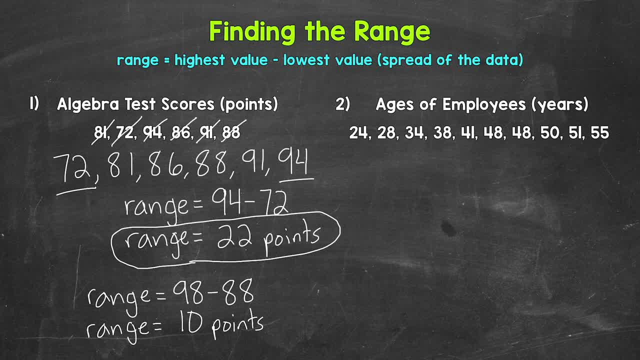 than the student above. that gives us an idea about the spread of that data. that data, the test scores, will be less spread out than the student above. and think about it: the above student, we go from 72 points to 94 points. that's more spread out.